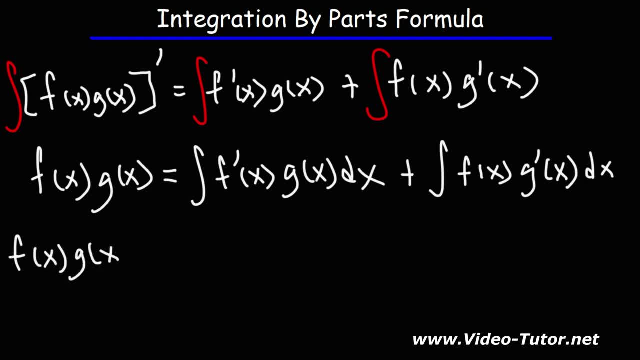 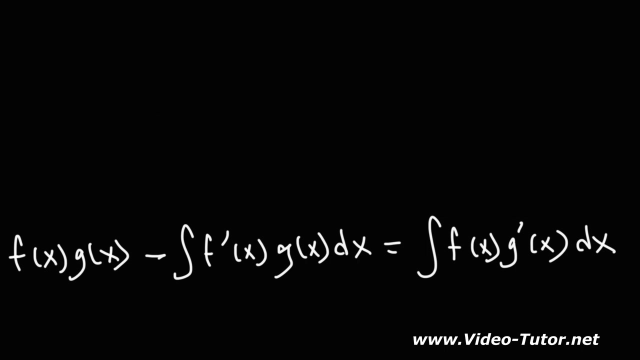 So I'm going to have f of x, g, x and then minus the integral of f prime of x, g, x, dx, And that's going to equal the integral of f times g prime. Now what I'm going to do next is is I'm going to reverse the two equations. 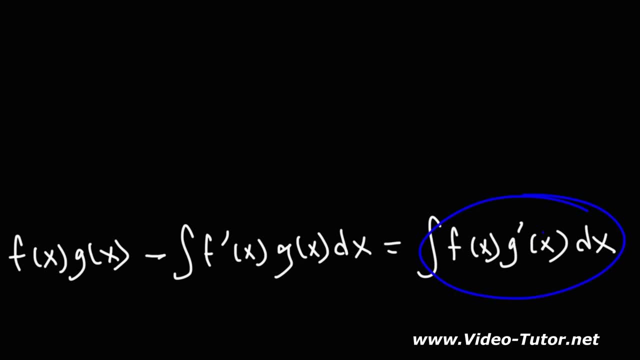 So I'm going to rewrite the right side on the left side and the stuff on the left side I'm going to rewrite it on the right side. So the integral of f times g prime is going to be f times g minus the integral of f, prime, g, dx. 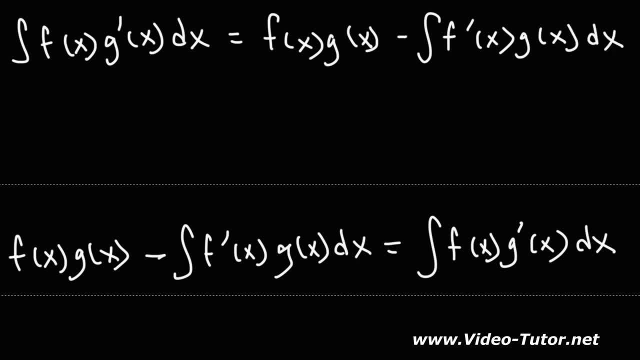 Now we're going to start introducing the u and v variables. Let's say that u is equal to f of x. If that's the case, then v will be equal to g of x. Differentiating both sides of that expression, u becomes du. the derivative of f of x becomes f, prime of x- dx. 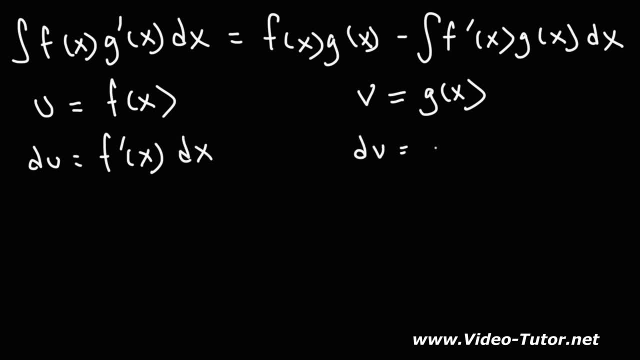 The derivative of v will become dv and the derivative of g of x will be g, prime of x, dx. So now let's replace what we have in this expression with u and v. So f of x, that's going to be u. 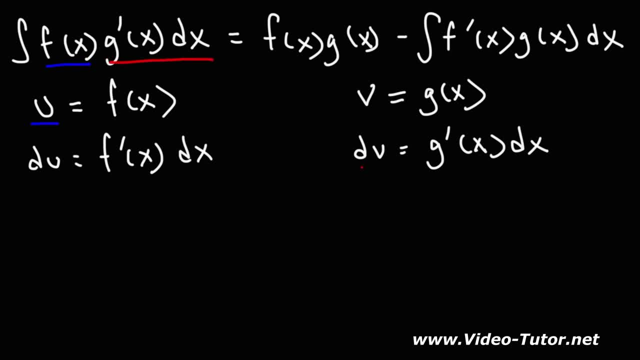 and g. prime of x dx will be dv. So on the left we have the integral of u times dv, and here we have f times g. f is u, g is v, so that becomes uv minus the integral of. so g of x is simply v. 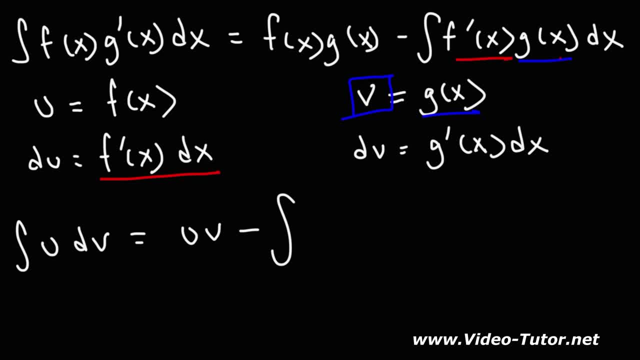 And f prime of x dx, which we could say is u, and g prime of x dx, so that becomes uv minus the integral of, so g of x is simply v And as you can see here, that's going to be du.